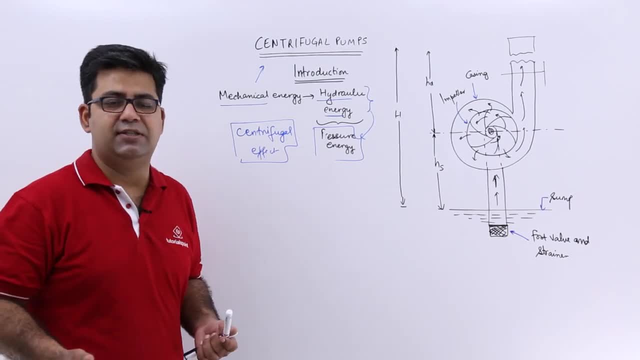 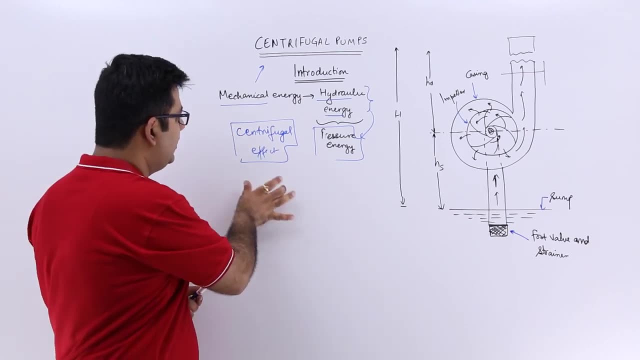 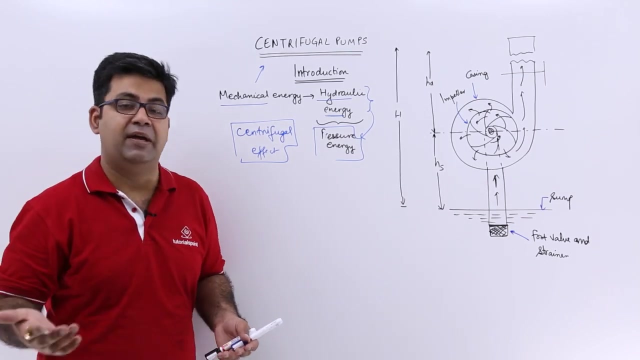 Okay, so in a simpler way, I would say that centrifugal pump is a pump. It converts the mechanical energy, with the help of the centrifugal effect, into the pressure energy In more simpler ways. if you remember the radial turbines, this is nothing but a reversed inward radial flow turbine. 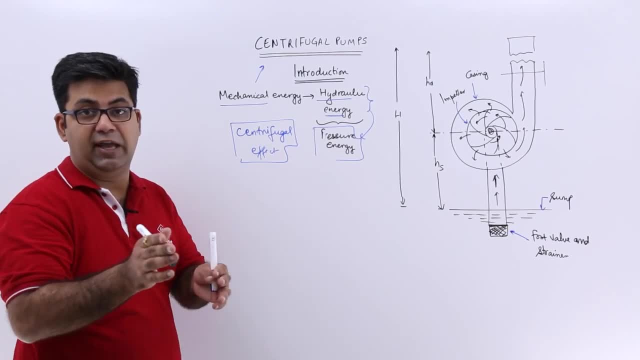 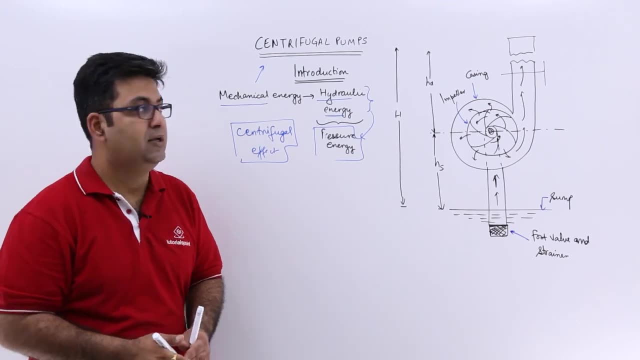 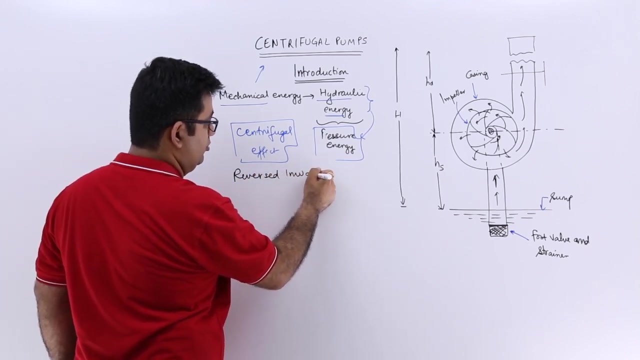 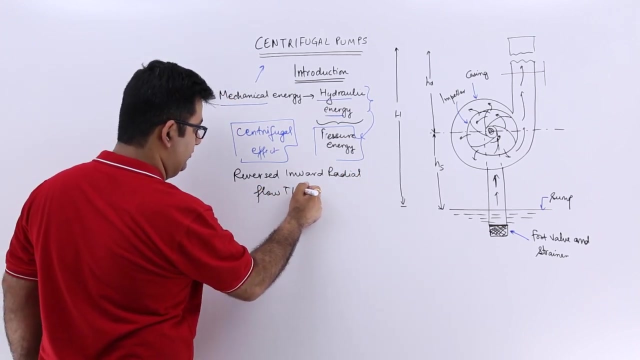 Reversed, not the actual one, because turbine is an energy producing device. pump is an energy consuming device, So this would be A reversed inward flow or I would say an inward radial flow turbine. Alright, So you can look at a centrifugal pump in this fashion as well. 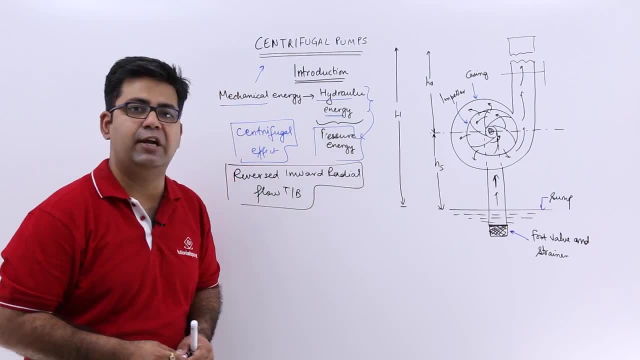 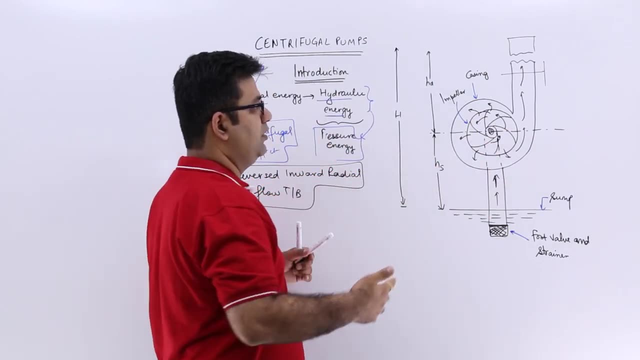 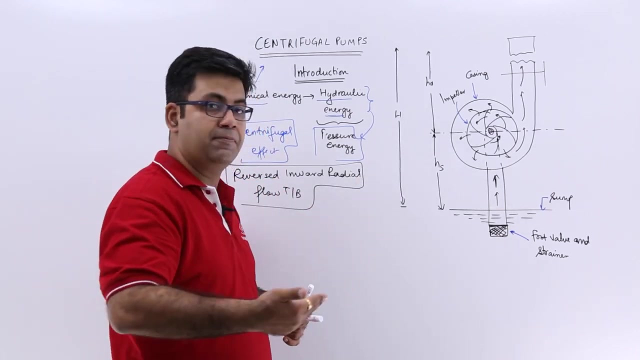 Alright, so this is the basic schematic of a centrifugal pump. The main components of a centrifugal pump are that you have an impeller which is somewhat like the runoff. You have an impeller in the turbines- Alright. so impeller is connected to the prime mover which rotates it, gives it mechanical. 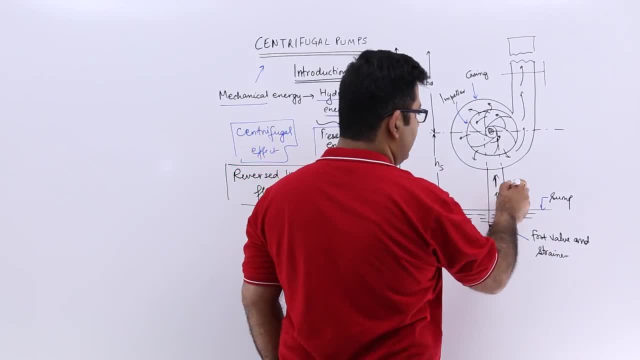 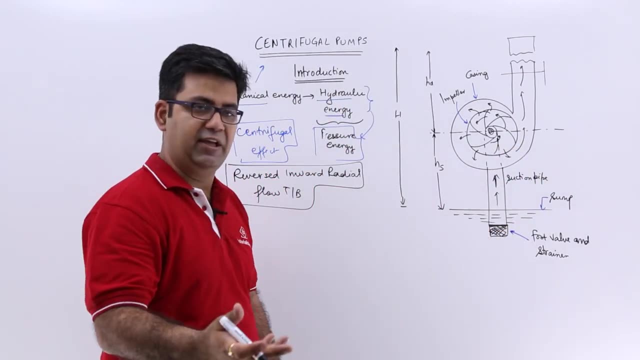 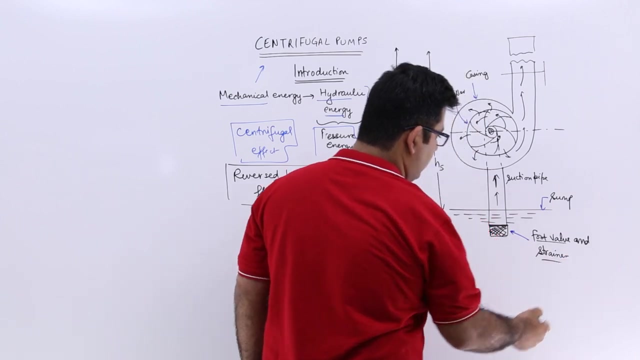 energy, okay, and then you have a suction pipe. suction pipe which goes down the sump, where the liquid is there which is to be pumped to a higher head. This is the foot valve in the strainer which separates all the, you know, impurities of. 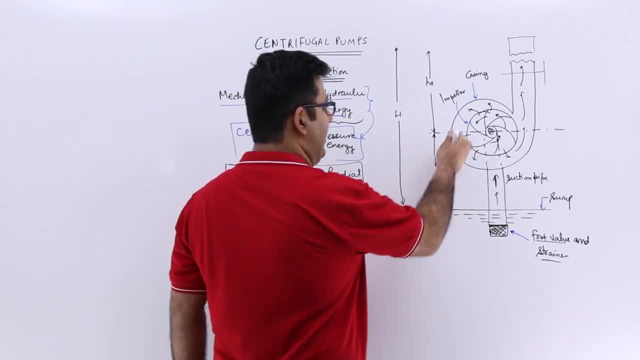 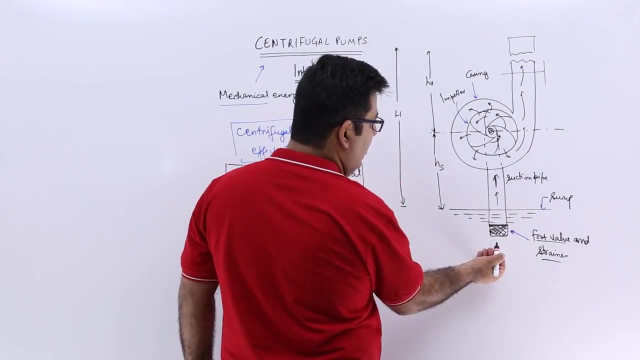 the pump. This is, for you know, hard particles to be entrapped inside these moving parts of the pump. Alright, so this acts as a filter. Then this is the sump. the liquid rises up the suction pipe, enters the impeller eye. 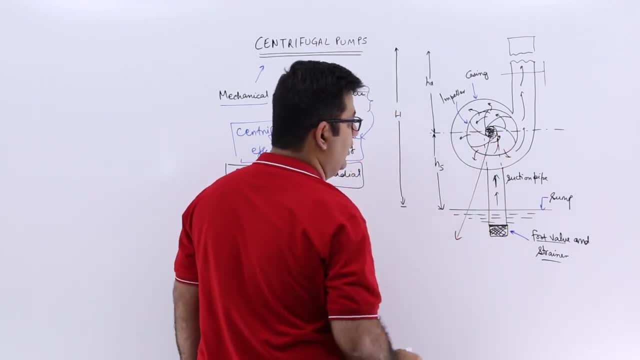 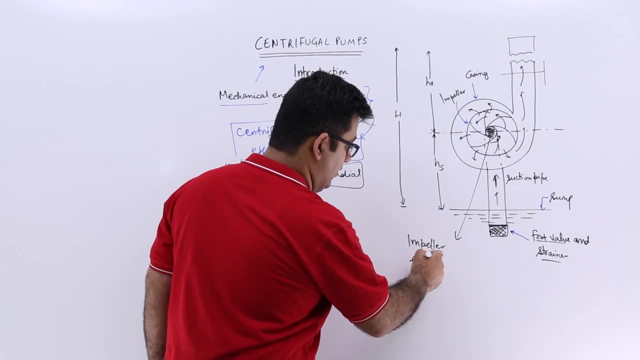 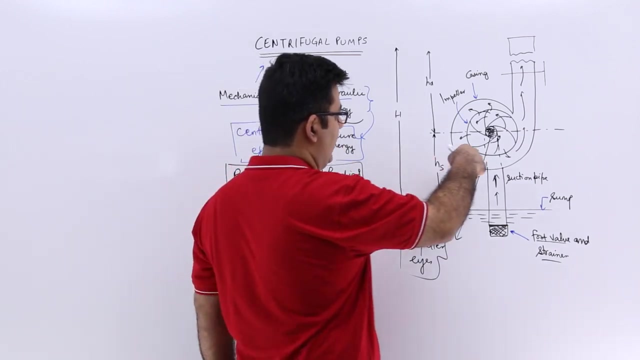 So this part, this part is called the eye of the impeller And this is where the suction happens, or the inlet is there for the liquid in the centrifugal pump. Then it rotates, comes out, collects in this casing. This is called the spiral or the volute casing.